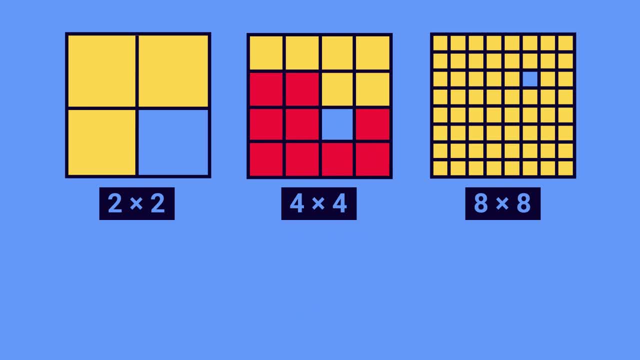 because for any given blank square, you'd have to try to tile the rest of the grid and hope it works, unlike this attempt that failed, and then you'd have to do this for every square being the blank one. So, in order to solve this, 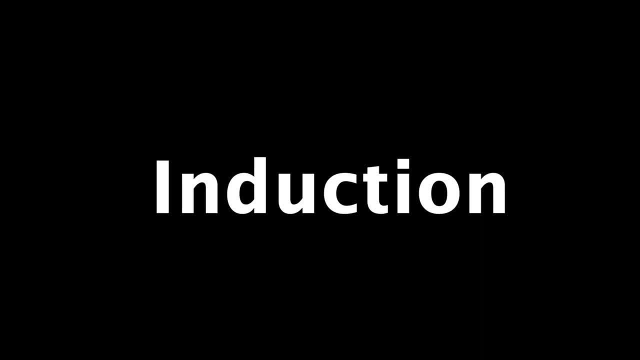 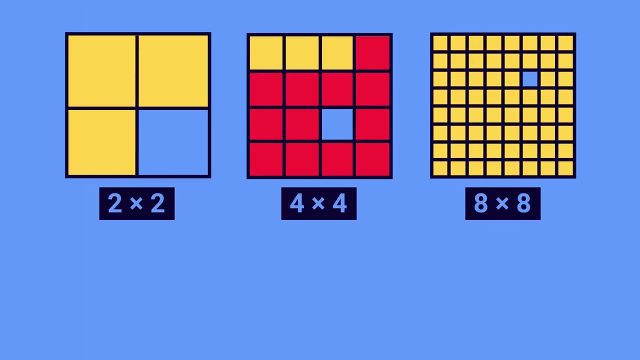 we're gonna use mathematical induction, which you need no real background to understand. Most schools and videos explain induction with classic examples that involve series and summations, but visual examples like this is what finally made me really understand the proof method, and that's all this video will include. 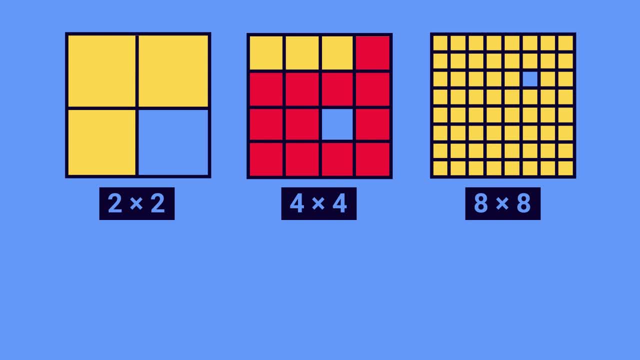 Now, induction is nice in that it just involves two steps, and the first is very easy. All we have to do is prove our assumption is true for the base case. often this is when n equals one. So n equals one here corresponds to a two to the one. 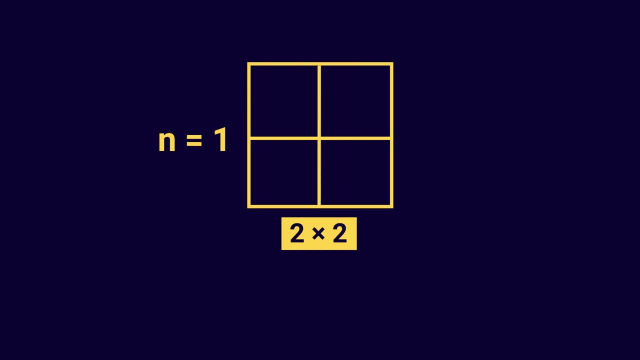 by two to the one grid, and it's easy to see. this can be tiled with L-shaped tiles besides one square, If I want this square to be the untiled one, then we just do this. If I want this square to be the one left open, 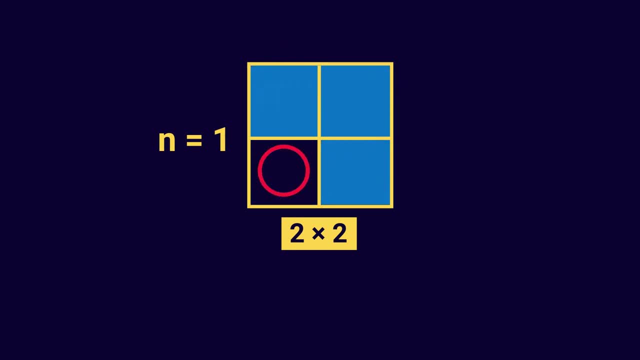 then we rotate the tile as shown and we can do the same thing for the other two. So I can tile this entire thing but leave any one square open. We now know this works for a two by two grid, or n equals one. 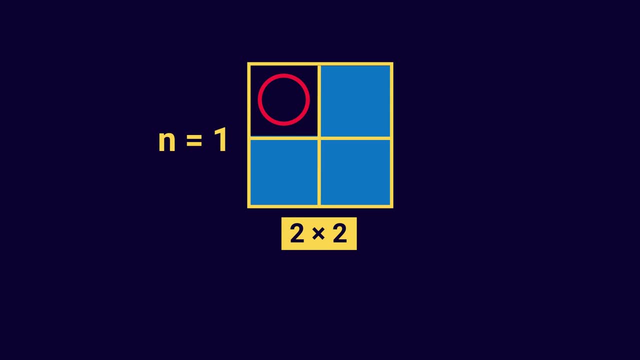 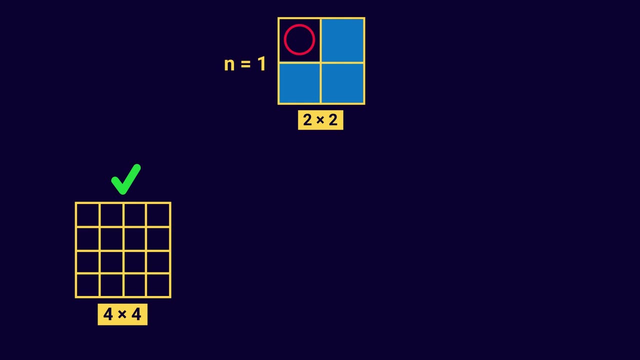 Now we just gotta prove it for every other integer value of n. The second step, though, is what confused me for a while. What you do is assume that our statement is true for any n. I'm putting a four by four on the screen, specifically. 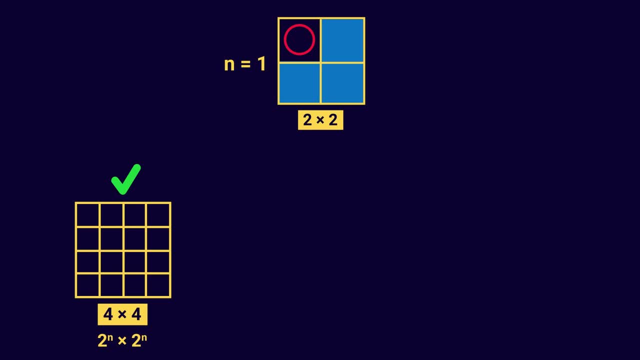 just to help with the visuals. but no, formally you just assume this is the case with any n. So for our example, we assume any two to the n by two to the n grid. besides, one square can be tiled, even though we have no idea if that's true. 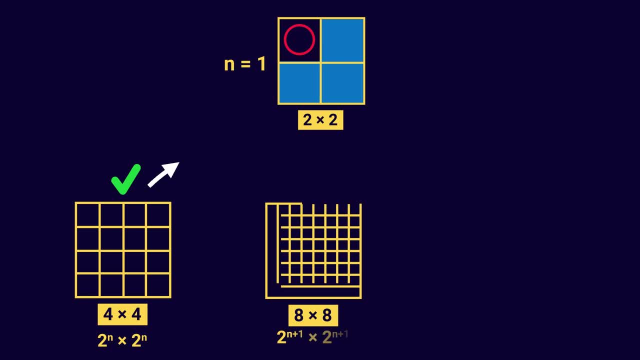 And then we have to prove that this implies we can do it for the n plus one case or the next largest case. If I can do it with a four by four, can I do it with an eight by eight? Or if I can do it with an eight by eight. 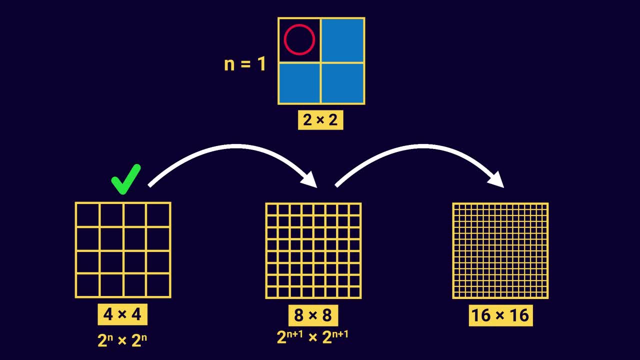 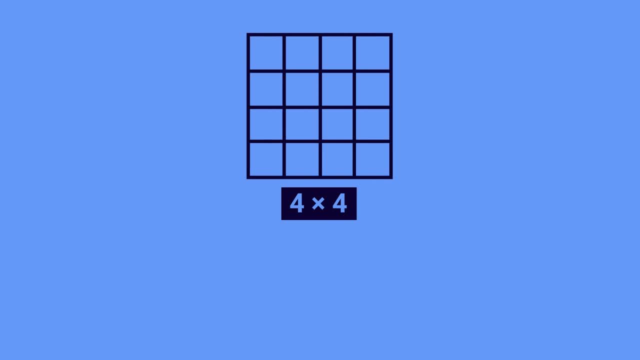 can I do it with a 16 by 16, and so on. We have to essentially prove all of these at once, So I'm gonna stick to the four by four and we're saying it can be tiled completely besides any one square. 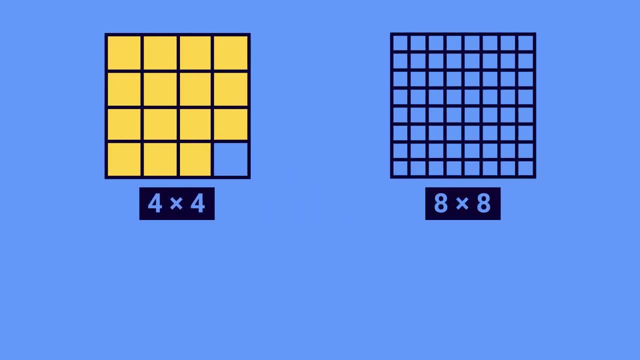 But does this mean we can do it with an eight by eight? Well, all we have to do is split that into four quadrants to get four different four by four grids. From the assumption we can say this grid on the top left can be completely tiled besides any one square. 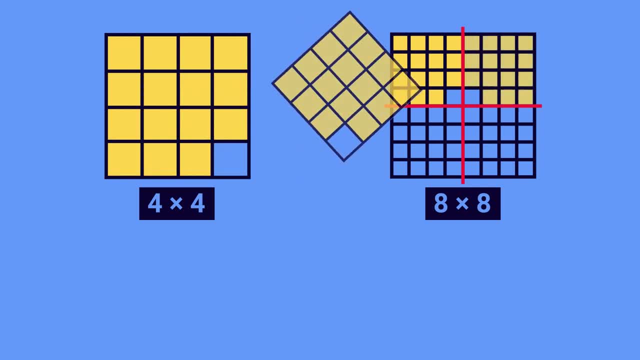 like the bottom right. This other grid can be tiled besides any one as well. we'll say the bottom left, And this one can be tiled completely besides any one like the top right. Then this last one. there's the untiled one. 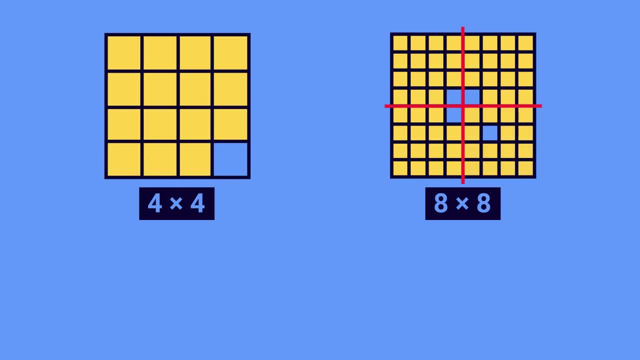 And I did it this way because, since this can be achieved with L-shaped tiles, based on our assumption, then one more here completes our task of tiling all but one square. This works for any blank spot, though If I wanted this to be the untiled one. 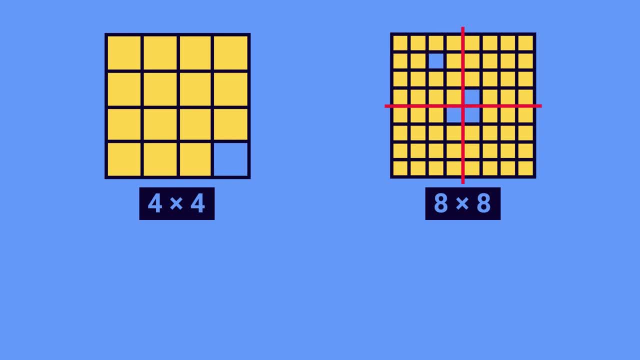 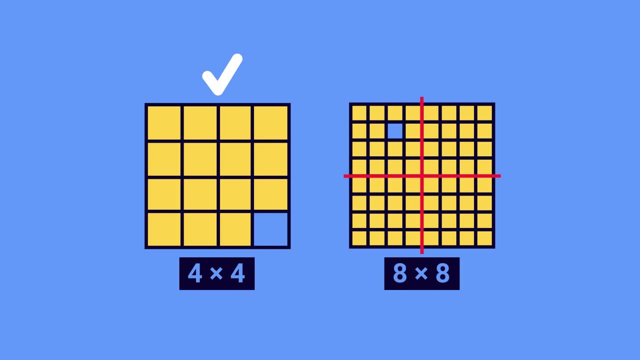 then we could just use the four by fours to complete the other three quadrants as shown and then fill in the middle again. So we've shown that if a four by four grid can be tiled as we want, then an eight by eight can as well. 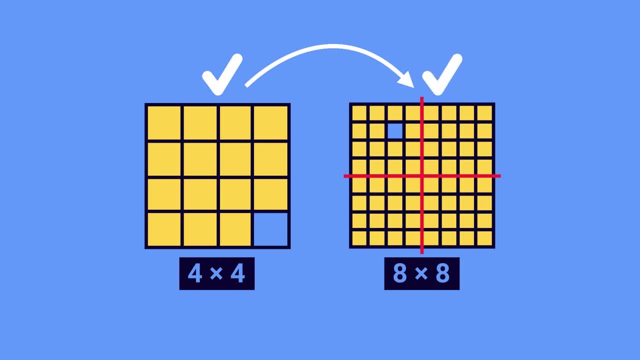 But this can't be done with an eight by eight. This keeps going Because if this works with an eight by eight, then it works with a 16 by 16, by just splitting it up into quadrants and filling in the middle spaces, like before. 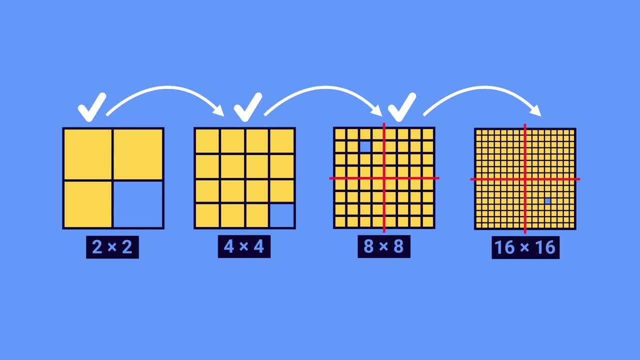 And going down. if a two by two grid can be tiled as we want, then a four by four can as well, with the same reasoning. But the two by two case we did prove that's the only one we actually know is true. 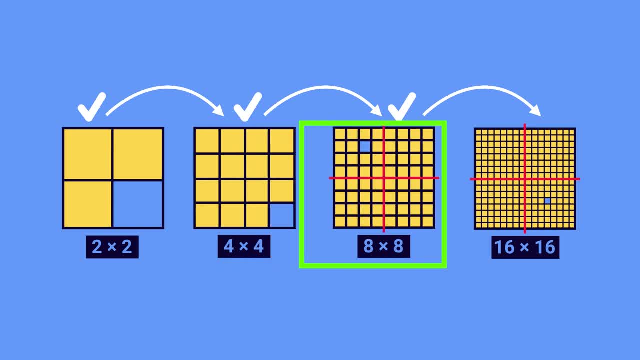 But now we know that means it works for the four by four, then the eight by eight, and so on forever. So we've proved what we wanted, that for all integer values of N we can tile the whole thing with L-shaped tiles. 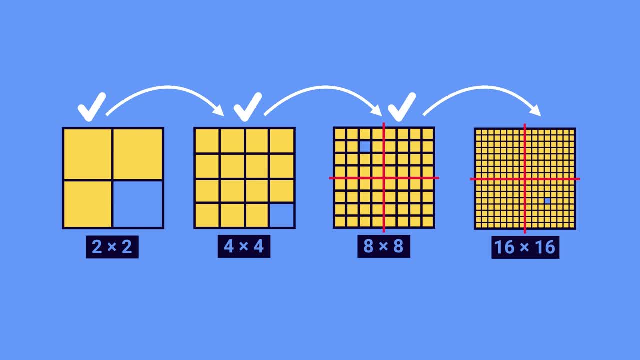 besides one square. This is not a formal introduction, by the way, as you won't really see all these specific values of N use, So just realize that. but I think it's easier for the visualization. Induction doesn't help us figure out these formulas. 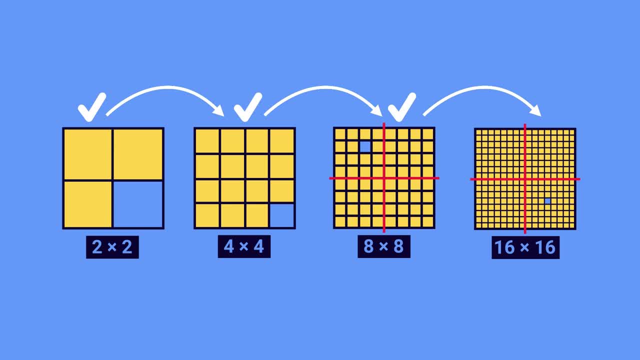 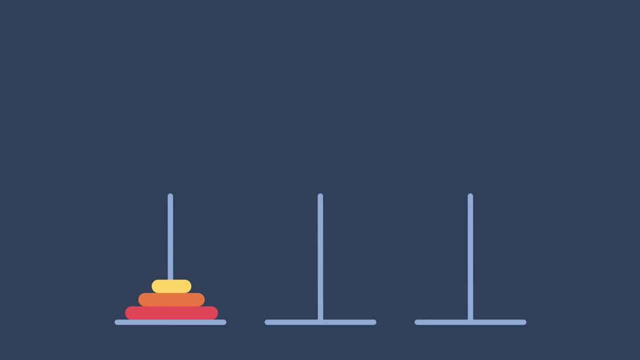 by the way, but it does help us verify them. Another example has to do with the Tower of Hanoi game. How this works is that you start with a stack of disks on the left rod, ordered by size from smallest, on top of the first. 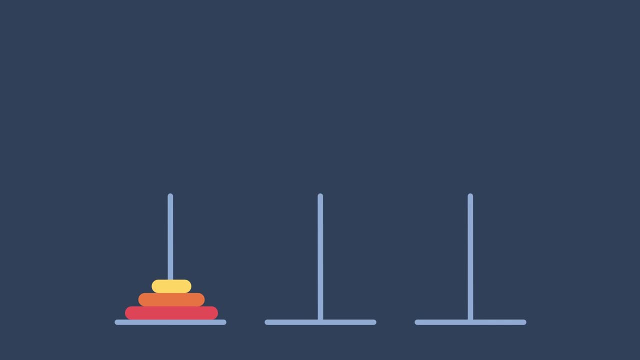 The goal is to get the entire stack to another rod, also in descending order. but you can only move one disk at a time. You can only move the top disk from one of the stacks and you cannot place any disk on top of a smaller one. 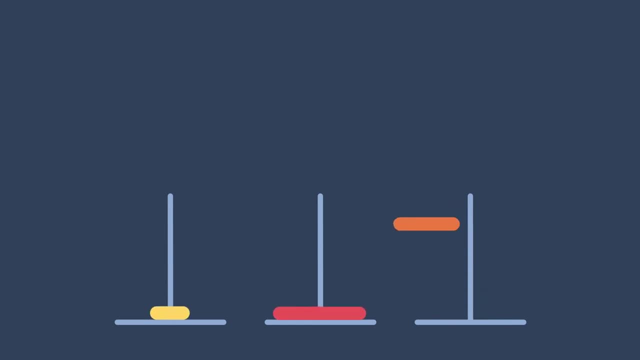 So this would be an illegal move, And I'll just complete the game where you can see now we have successfully moved the stack to a different rod. The goal is to prove that the minimum number of moves this game takes is two to the N minus one. 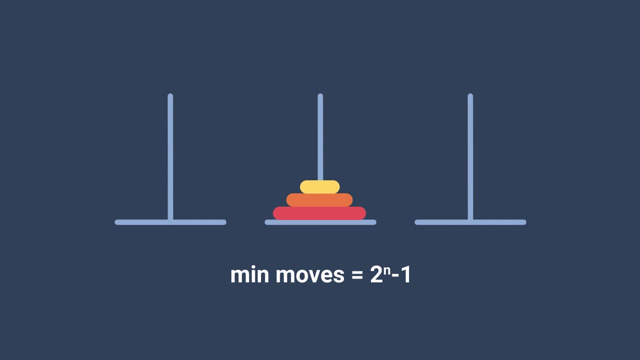 the number of disks. Well, to do this with induction, the first step is the base case. If N equals one AKA one disk, plug that in and we find it should take one move at the minimum, which is obviously true. 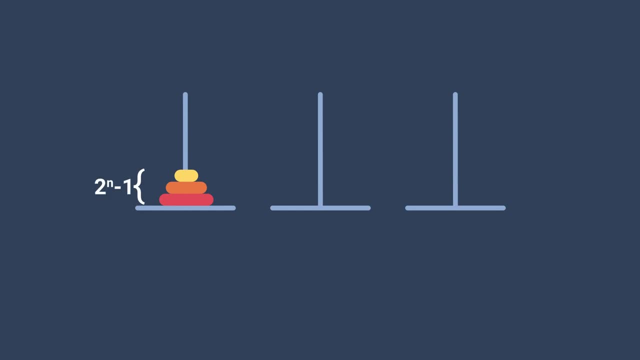 Now for the next part. we're gonna assume this formula is true for some arbitrary number of disks and the goal is to prove that this implies the expression works when we add one more disk. Remember, we're proving this for basically all values of N at once, because once that's done, 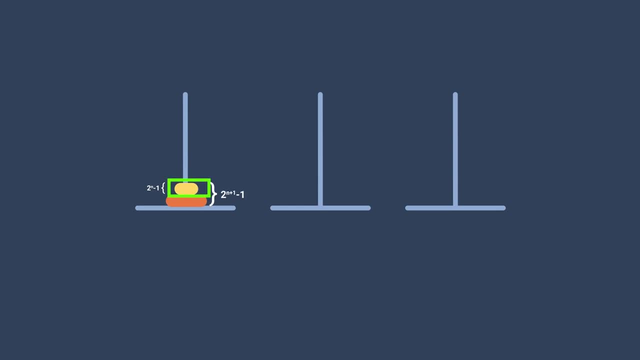 the fact that we already have the base case will imply that two to the N minus one works for N equals two, which will apply to N equals three and then four, and so on forever. Now for the proof. we've assumed, at minimum: 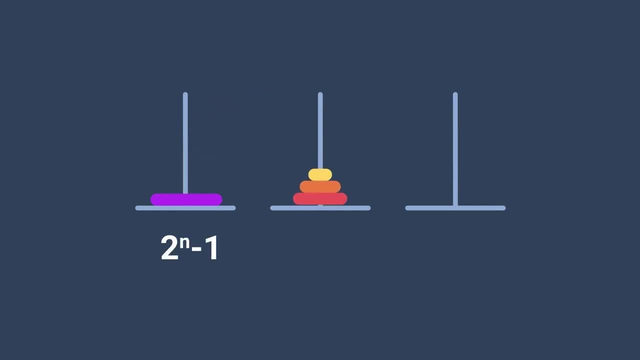 it'll take two to the N minus one moves to move those first N disks from the left rod to another. It then takes one move to put the largest disk on the empty rod, and again it takes two to the N minus one moves to move that same stack of N disks to a different spot. 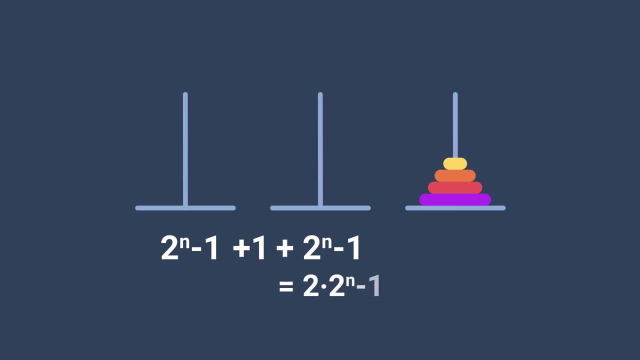 If we combine all these expressions we get this here and the two times two to the N is just two to the N plus one. So if it takes this many moves at the minimum for N disks it means the formula works when we add in another disk. 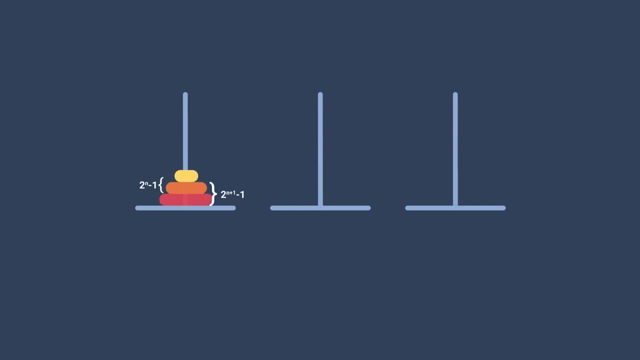 And since again we know it works, for N equals one, then two to the N minus one applies to every value of N, And I'll show one more example, because this one's pretty clever. The goal is to prove that a circle can be divided. 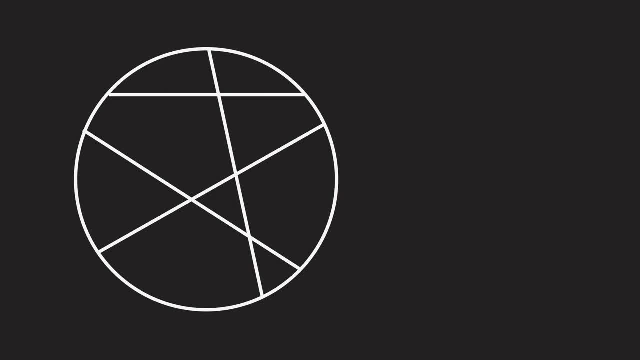 into regions by any number of line segments N, and be colored with just two colors, such that any two regions that share an edge like these two have different colors. Obviously, we're gonna use induction here and the base case, or N, equals one. 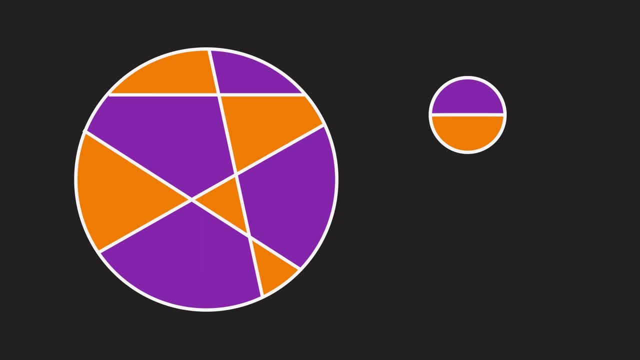 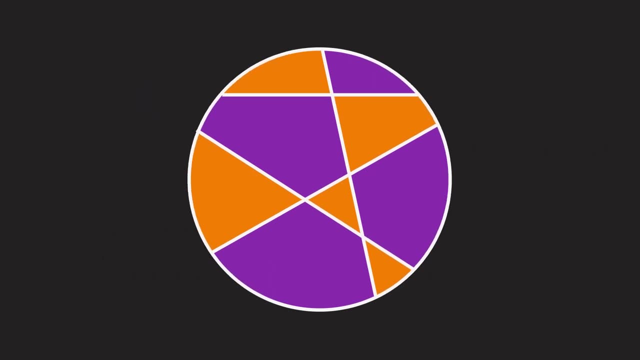 corresponds to a single line segment. No proof is really needed here, because obviously this can be two colored. But now we gotta assume that it is true for any number of line segments and prove that. and prove that this implies that it's still possible. 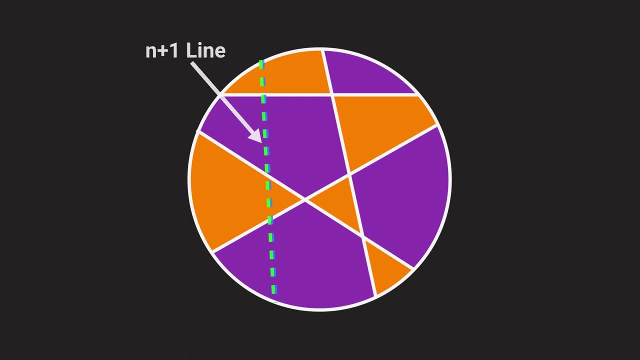 when we add in another line. Now again, I'm saying N lines, but I'm using four here just for simplicity. And although we are seeing that, yes, it can be two colored, that's just for the visuals. We don't know that for sure. for any N. 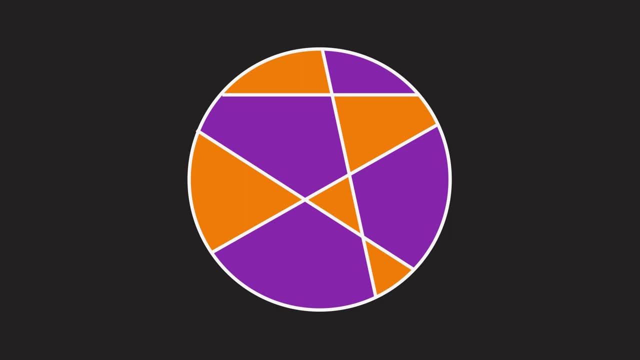 besides, N equals one right now. But this second inductive step is probably the least obvious of all the examples we've seen in this video. I mean, how does the fact that this can be two colored imply that this can as well? Well, that last line we drew divides the circle. 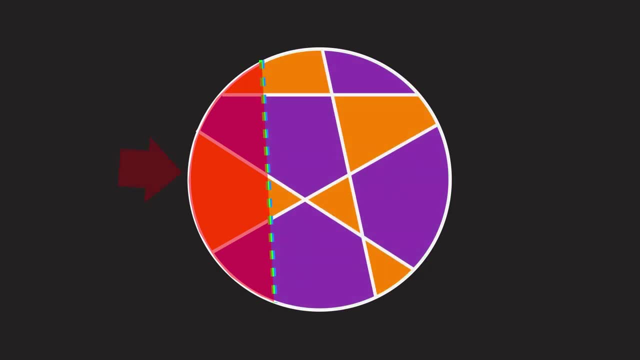 into two regions, and if you take all the little regions on one of those sides and invert the colors, you get a circle that is successfully two colored. Here's why that works. Let me put back the previous configuration When we add the extra line segment. 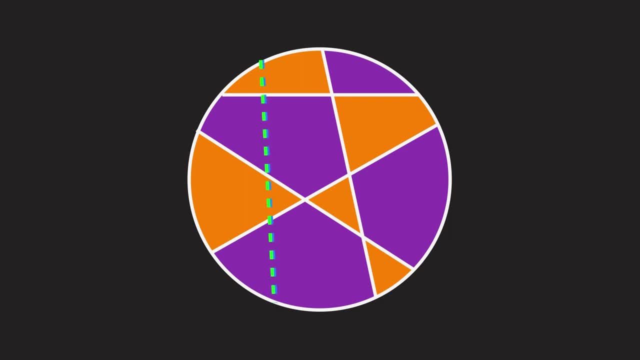 then any two neighboring regions in this newly partitioned circle will come in one of two categories. First is that there's shared edge, and then there's two, And we know that their shared edge is not a part of that new line segment. So like these two or these two, 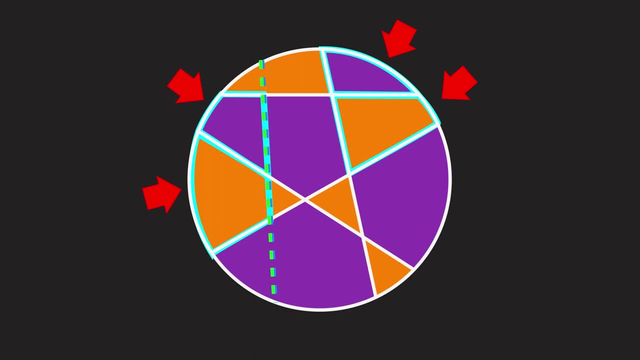 their shared edges are not part of the dashed line. Since that's the case, they're guaranteed different colors already from our assumption, which means leaving them alone, like I'll do for the ones on the right, or swapping the colors of both. 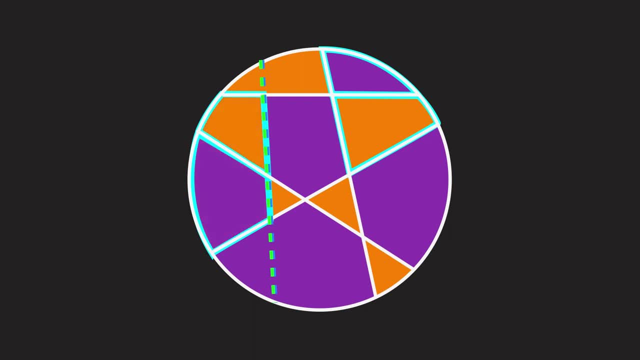 which I'll do for the ones on the left- still satisfies the two coloring condition. at least for those specific regions, And regardless of how the circle's divided, this will work. The other scenario we have to consider is when two regions share an edge. 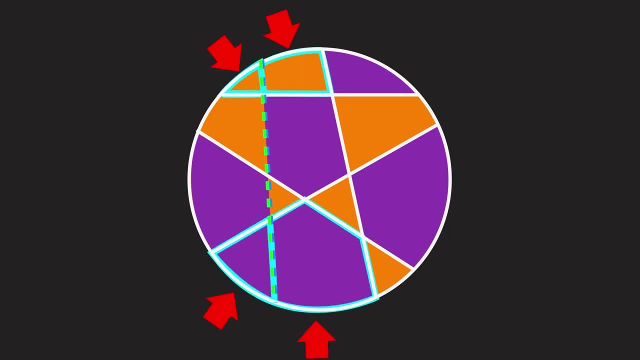 that is part of that line segment. like these two or these two, Those will be the same color at first, because the two coloring assumption was for the circle without that dashed line. But again our method was to flip the colors just on one side of that line. 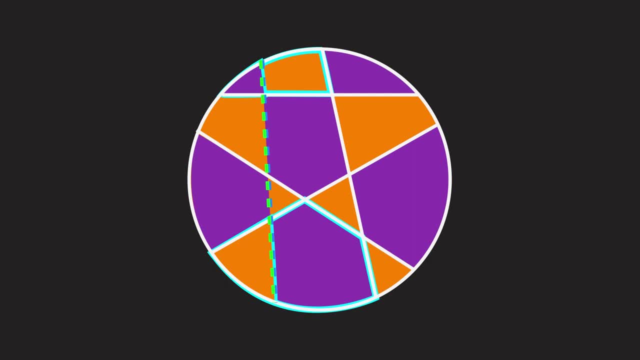 and that will fix the problem. making it so, the entire circle is now two colored. So we've proved that if the two coloring works with some number of line segments, it will work with one more by just inverting the colors on one side. 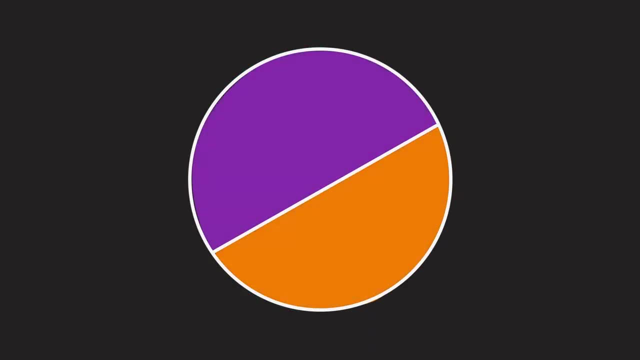 And since we know the two coloring always works with one line segment, then that means it works with any two, And that means it applies when we add a third and then a fourth, and so on forever. Thus, the two coloring will always be possible. 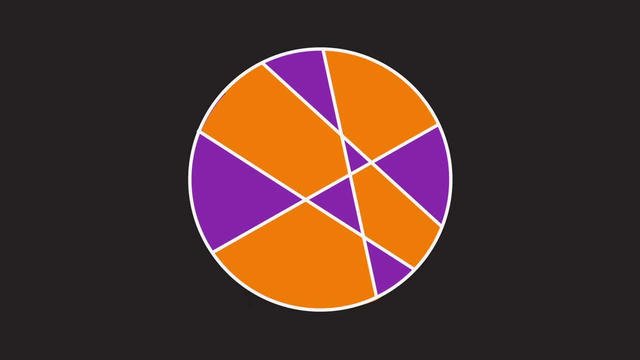 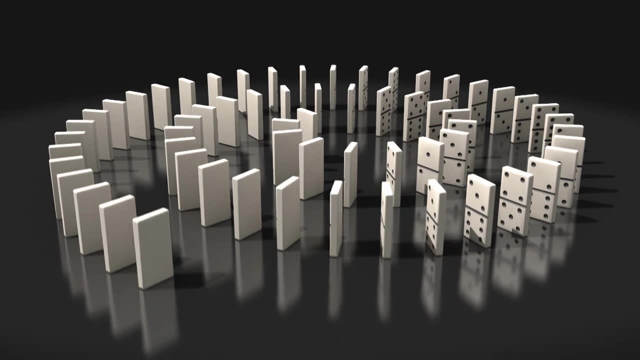 Probably the most famous visual for induction is dominoes being knocked over, where the second step, or the inductive step, is like saying that every domino is close enough to the next, or if one falls, then the next one will as well. 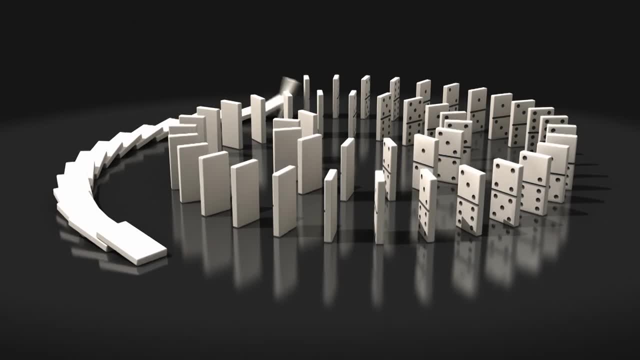 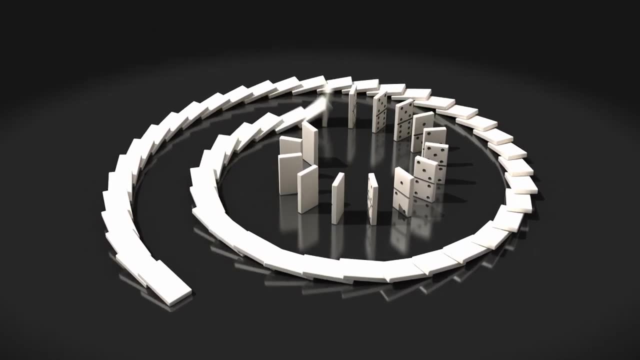 Any n implies n plus one, And the base case says the first domino got knocked over. so combine these two ideas and it must mean all the dominoes fall over. It's a good visualization, but hopefully these examples gave some more insight. 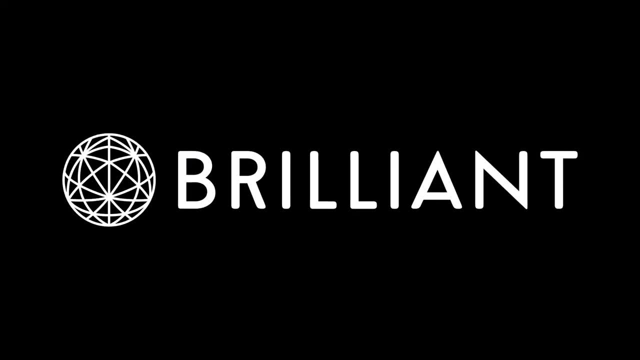 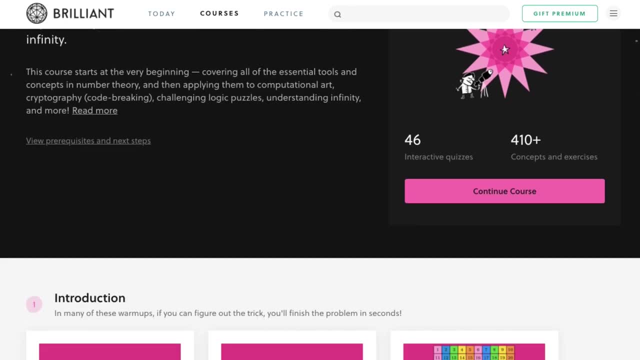 And for those who wanna continue learning cool math stuff, then I recommend checking out brilliantorg, the sponsor of this video. If you're interested in discrete math similar to what we've seen here, you'd enjoy their number theory course, which includes cool puzzles. 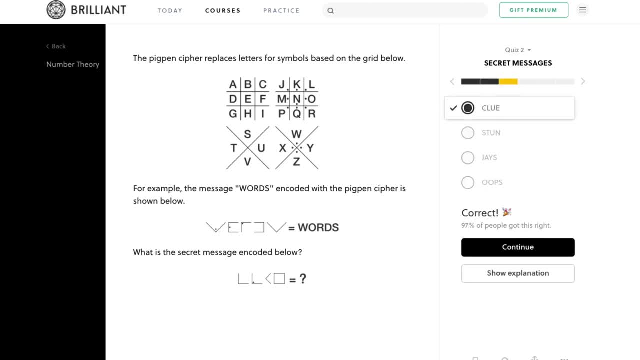 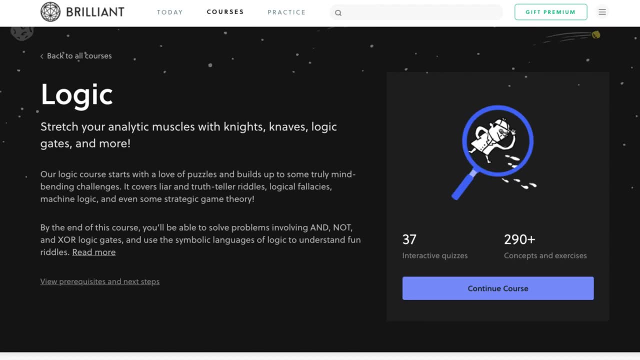 an introduction to modular arithmetic, the concept of infinity and much more. Or, for the pure math students out there, they have multiple courses in logic that'll challenge you with logic puzzles and simply introduce you to mathematical logic, which is a big prereq that sets you up. 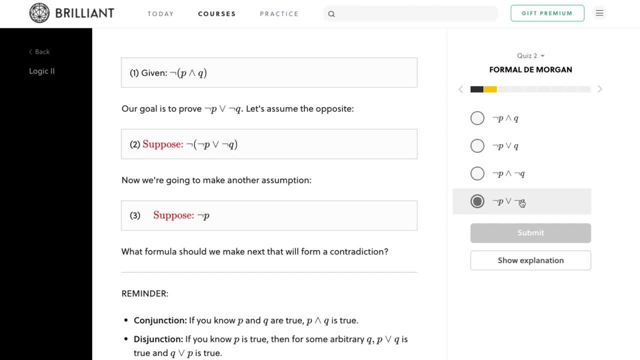 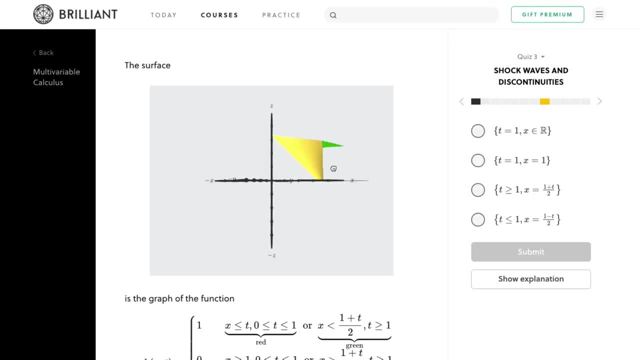 to take more upper level pure math courses in college. All brilliant courses come with detailed explanations, intuitive animations and constant practice problems to ensure you understand the fundamentals before moving on. For those who want to invest in enhancing your math or science skills for this new year, 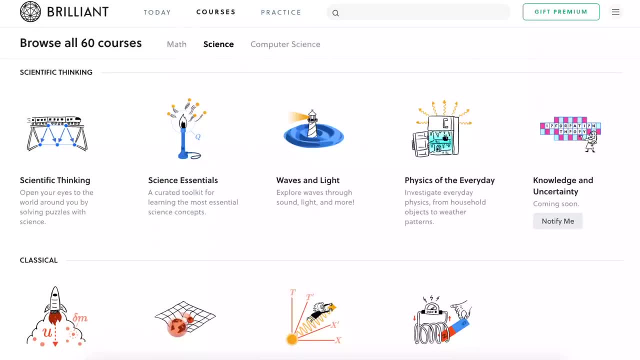 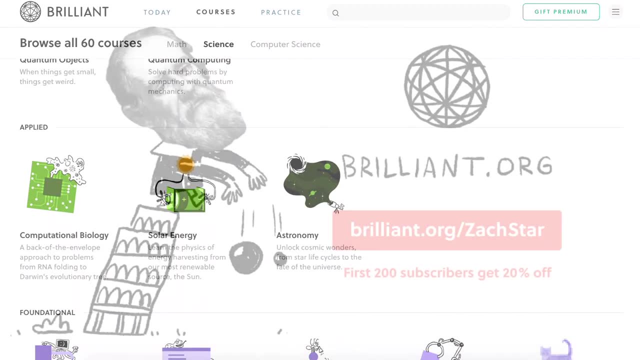 whether it be calculus, differential equations, group theory, astronomy or dozens of other topics. Brilliant has exactly what you're looking for, Plus the first 200 people to sign up by using the link or going to brilliantorg slash Zach Starr will get 20% off their annual premium subscription. 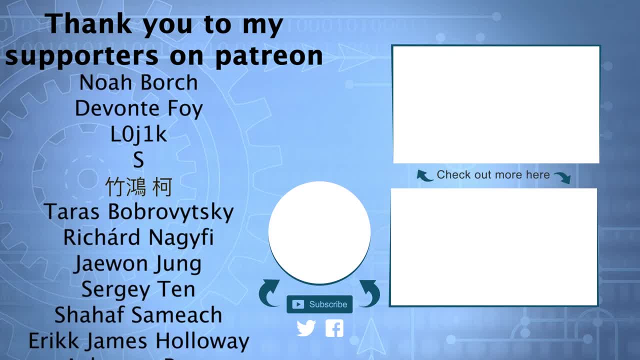 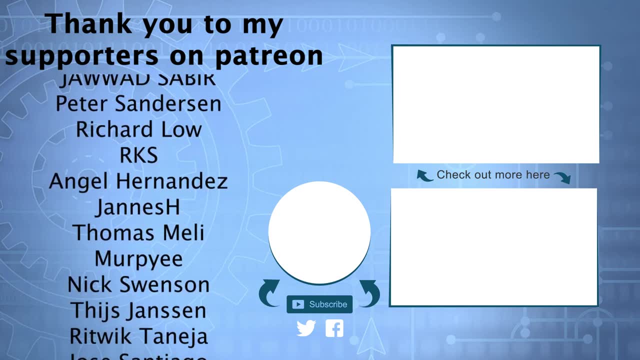 And with that I'm gonna end that video there. Thanks as always to my supporters on Patreon. Social media links are down below- and I'll see you guys in the next video. Bye.